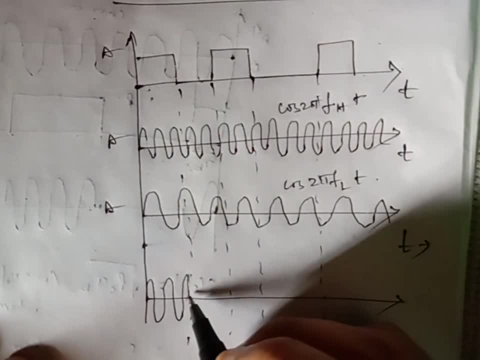 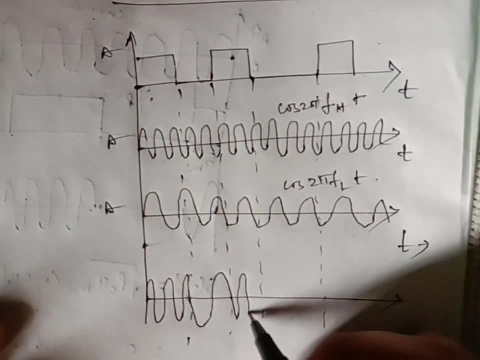 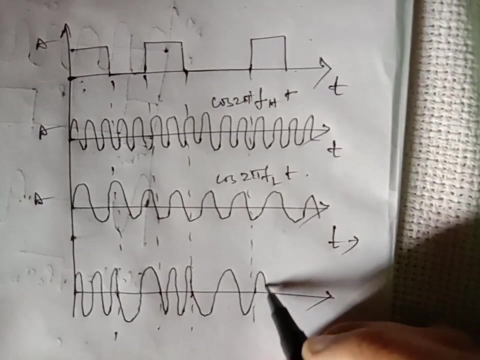 the carrier having lower frequency will be there in the output. So like this: Again there is one higher frequency, Again there is zero lower frequency, Again one higher frequency, Again one higher frequency, Again one higher frequency. So this is the waveform of BFSK. 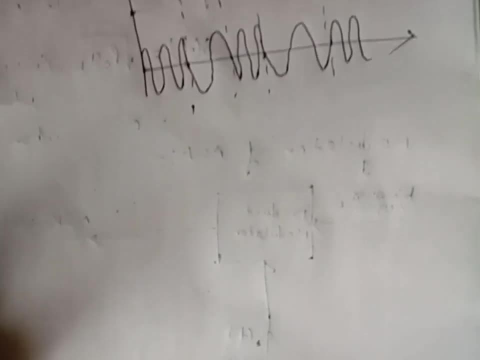 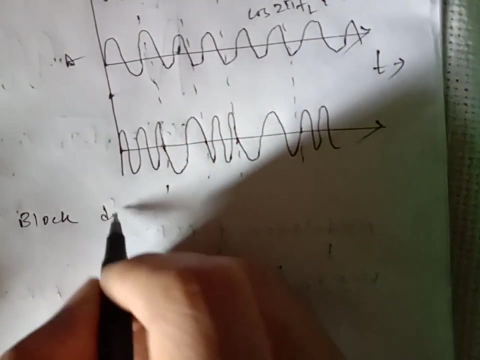 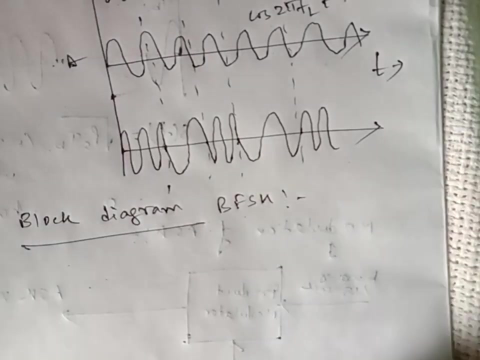 So now I will draw the block diagram of BFSK. Block diagram. Let this be the binary input sequence. bt 500 k devices. This is its input sequence, So which diag is obtained as the error? 0.. 0.. 0.. 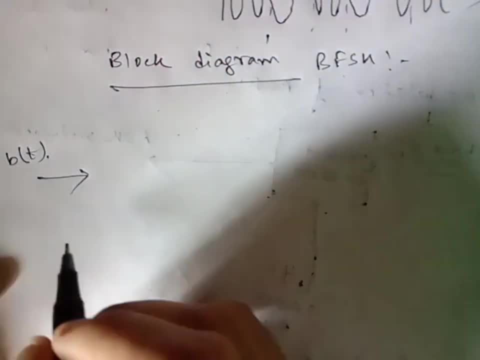 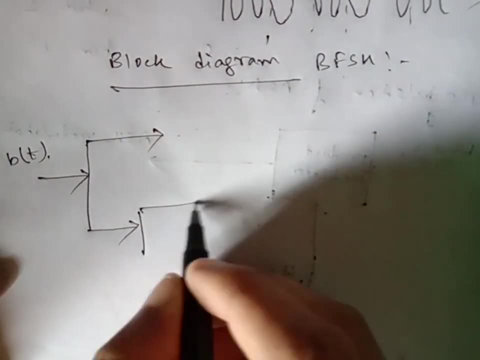 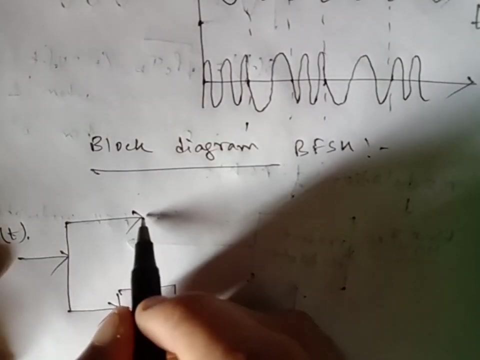 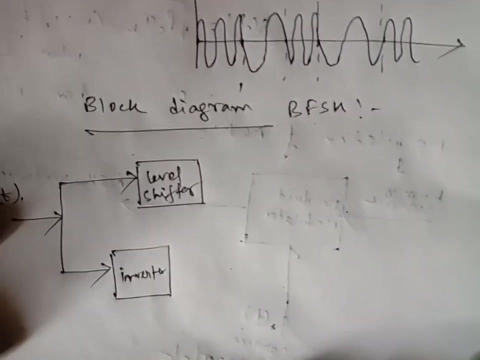 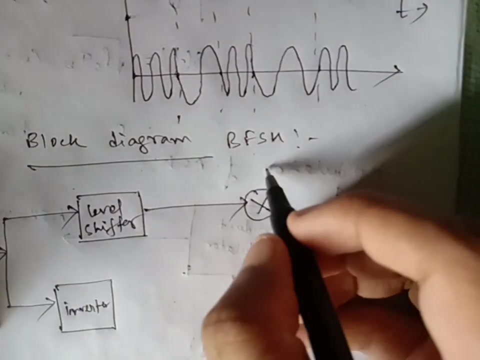 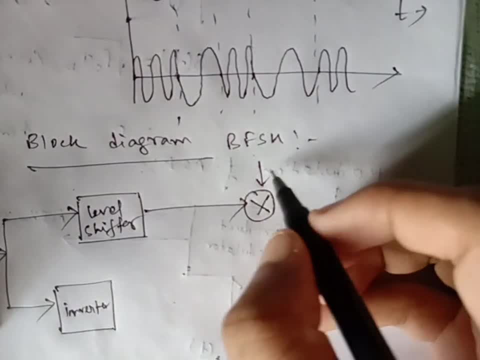 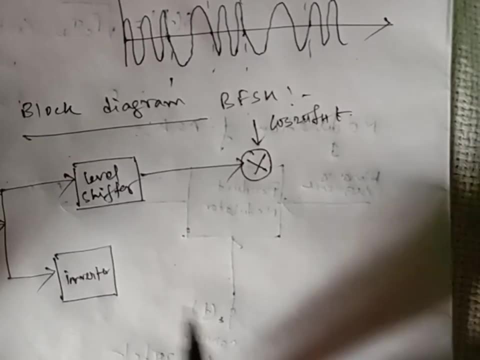 of the level shifter and the carrier having higher frequency, called 2 pi FHT. This output of the level shifter is given to two parts. one is given to a type ş, which are twoカンタ m. sinehelp is given to a frequency as the vaporized. 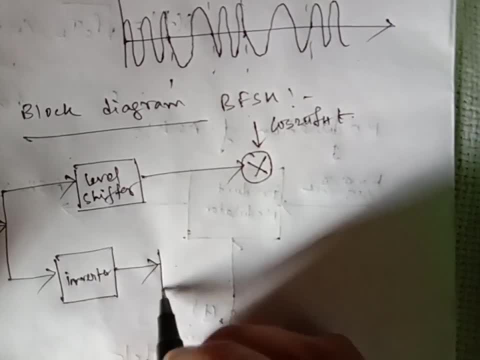 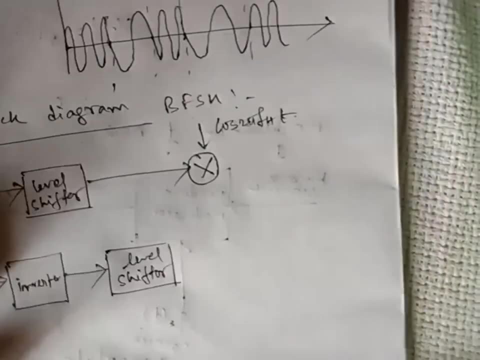 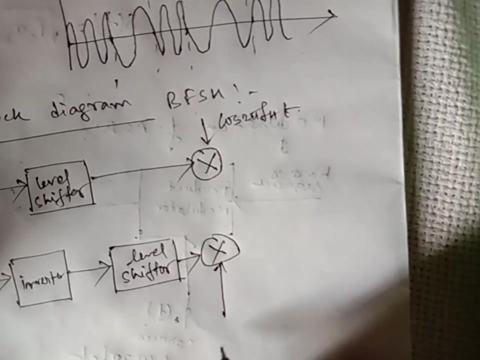 wafer in the liquid of the inverter is then passed through a level shifter and this output is again fed to a product modulator where the input is given as the lower frequency carrier, cos 2 phi, fl, t. one input is this level shifter, another input is cos 2 phi. 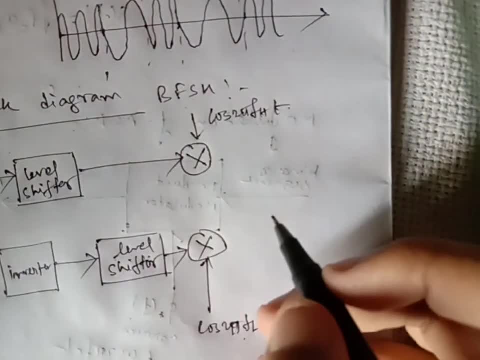 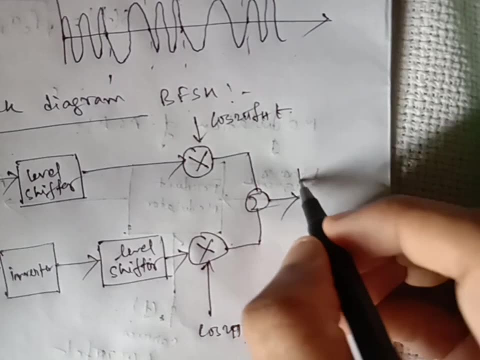 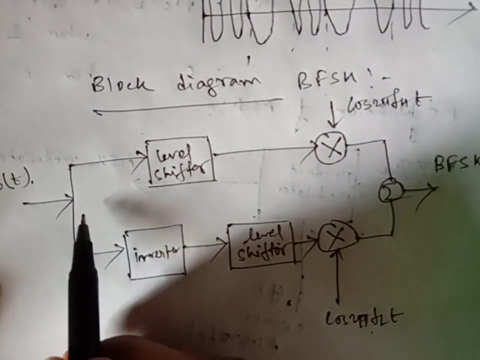 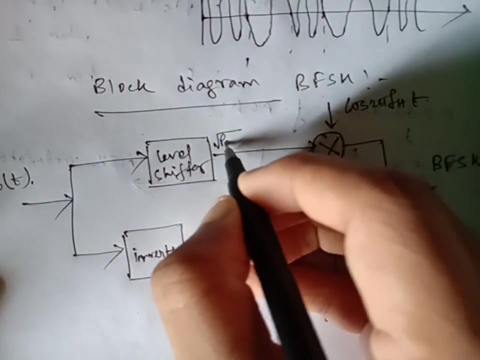 fl t, that is a lower frequency carrier, and this two output is summed and we get our resultant b fsk. so how it is working here, the binary input sequence, one part is directly given to the level shifter. so after the level shifter it will be like p s t b into p h t, right.